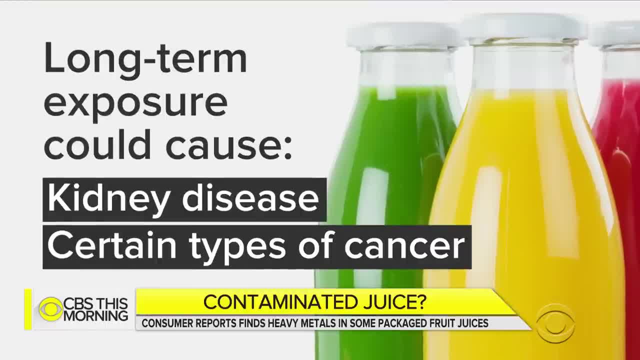 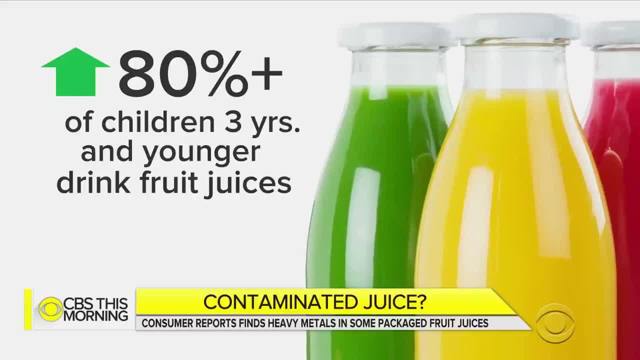 some serious health risks, like kidney disease and certain types of cancer. More than 80 percent of parents with children three years old and younger give their kids fruit juices. Anna Werner looks at what parents should do. Anna, good morning, Well, good morning. Heavy metals are substances that make. 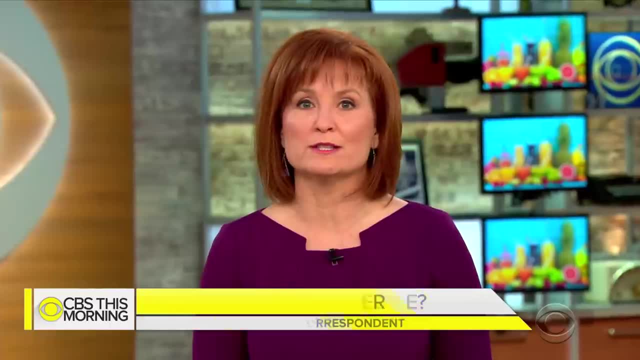 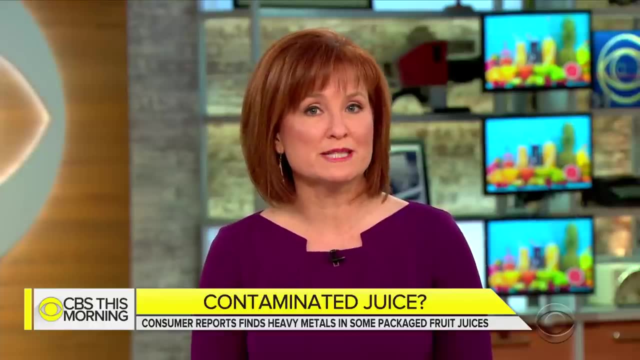 their way into food because they occur naturally in the air, water and soil. They can also wind up in food during the manufacturing and packaging processes. Now Consumer Reports says improvements have been made since they last tested juice products eight years ago, but they're still. 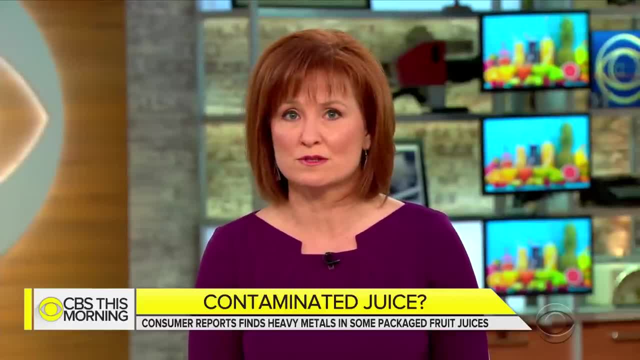 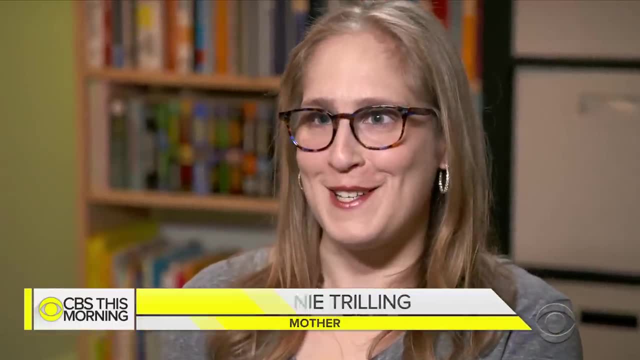 recommending that parents give their children less juice. As a mom, how do you think about fruit juice? So it's the bane of my existence. Sure, can you use your fork, Mom, Stephanie Trilling says she tries hard to keep her. 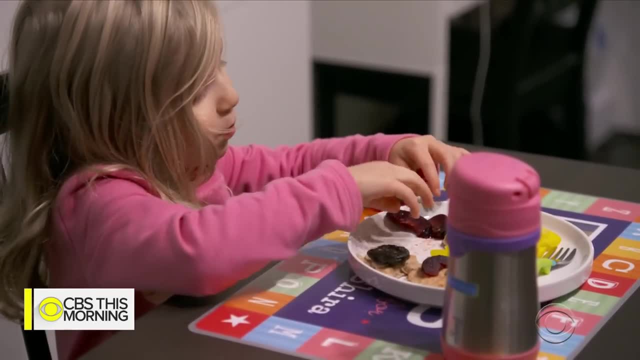 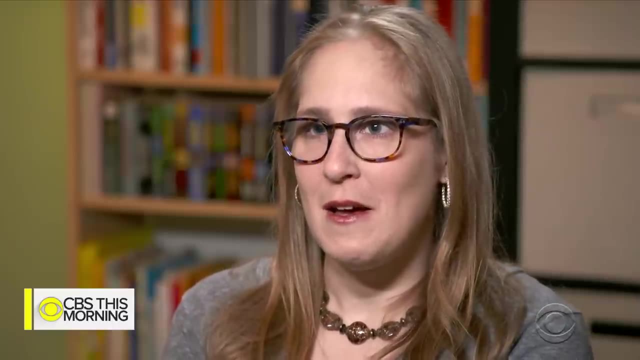 four-year-old daughter away from juice, mostly because of its sugar content. I'll be at a birthday party and I'll see it on the table and I'll cringe a little inside because it's not something I want to give to my kids. but I also don't want to be that mom who's 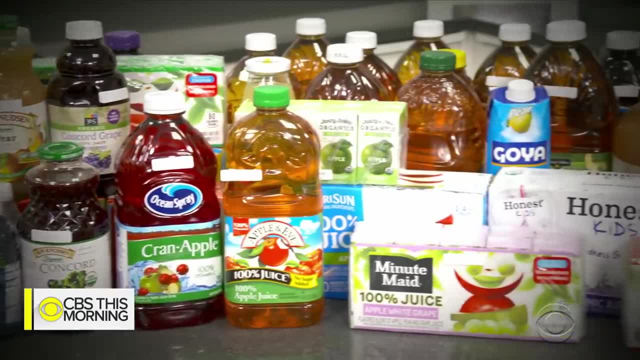 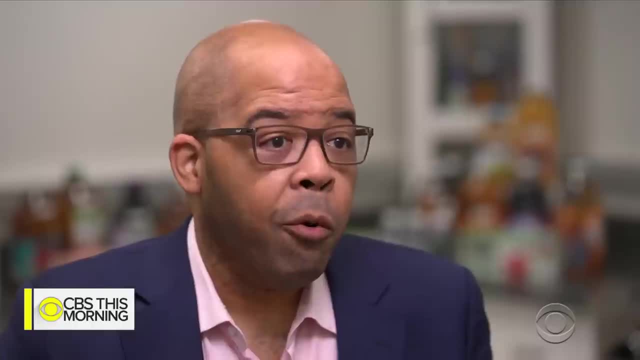 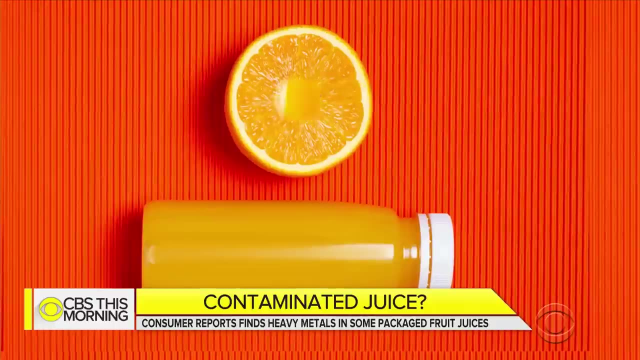 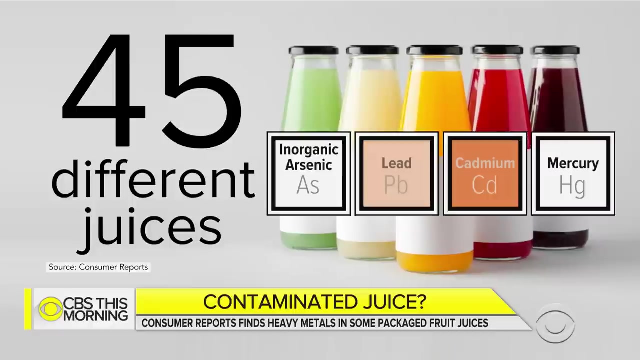 restricting everything. But she may have another reason to restrict juice intake: A new analysis from Consumer Reports. James Dickerson is chief scientific officer. Consumer Reports wanted to investigate the state of the juice industry, particularly bottled juice. His team tested 45 different juices for four heavy metal substances: inorganic arsenic, lead, cadmium and mercury. 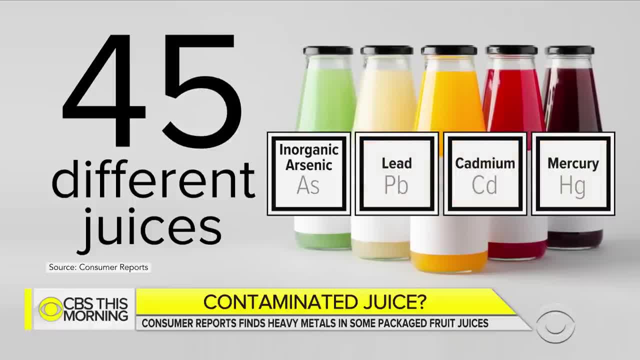 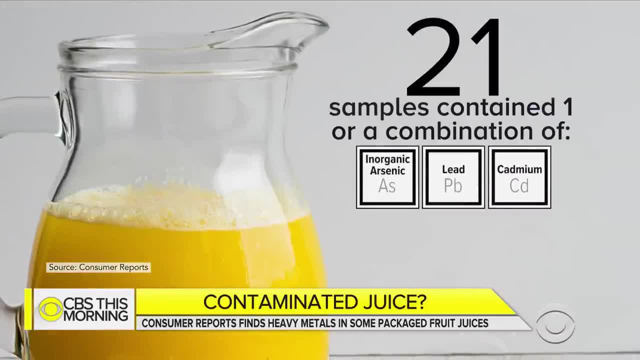 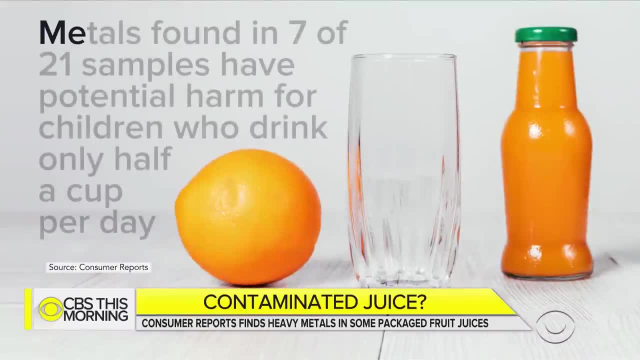 They found that every single product contained a measurable amount of at least one heavy metal, except for mercury. Twenty-one of the samples contained one combination of heavy metals that reached a level Consumer Reports researchers deemed concerning for daily consumption, And Consumer Reports says the metals found in seven of the 21 samples. 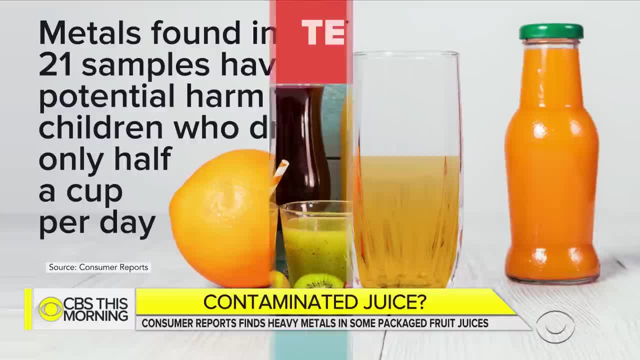 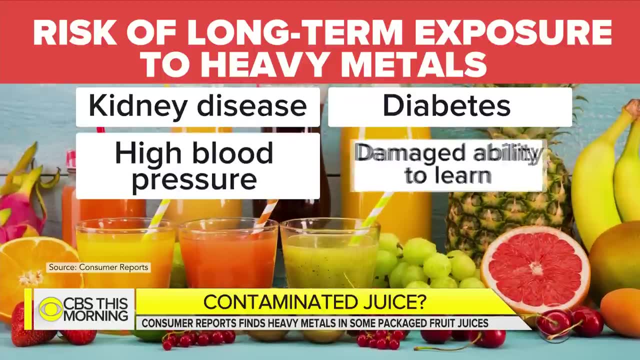 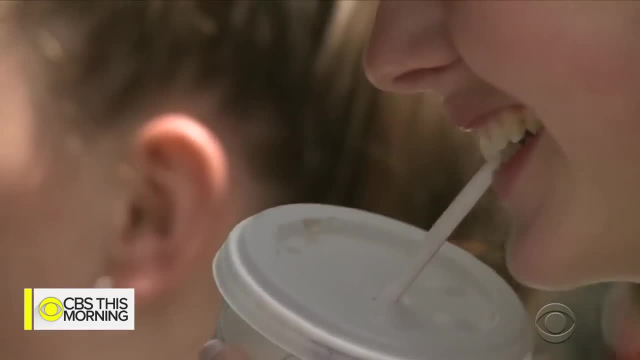 had the potential to harm children, who drink only a half cup per day. The CDC says long-term exposure to heavy metals may put people at risk for kidney disease, diabetes, high blood pressure, damaged ability to learn and certain types of cancer. Consumer Reports is recommending parents. 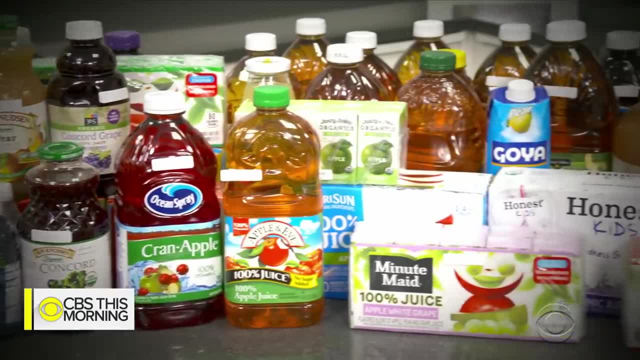 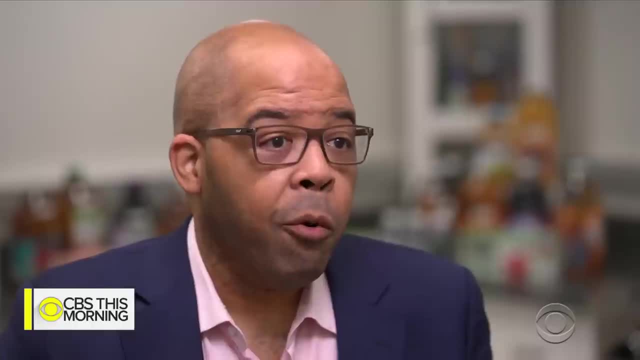 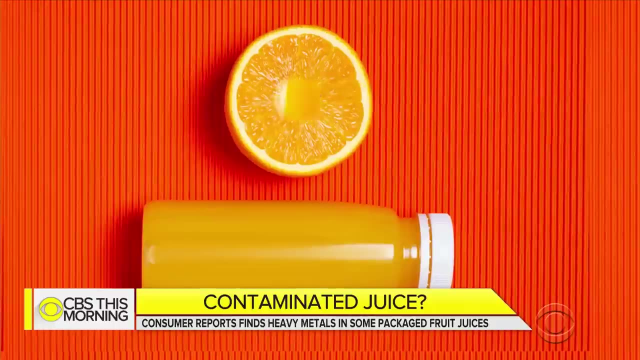 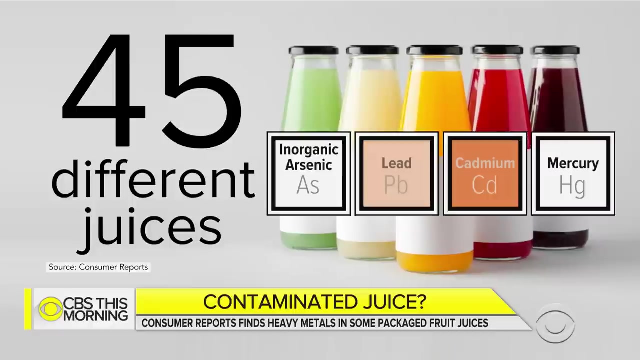 restricting everything. But she may have another reason to restrict juice intake: A new analysis from Consumer Reports. James Dickerson is chief scientific officer. Consumer Reports wanted to investigate the state of the juice industry, particularly bottled juice. His team tested 45 different juices for four heavy metal substances: inorganic arsenic, lead, cadmium and mercury. 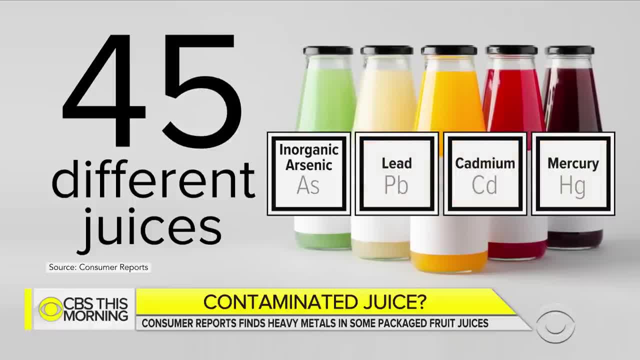 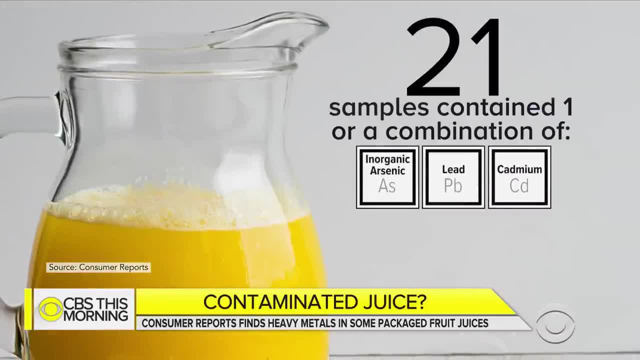 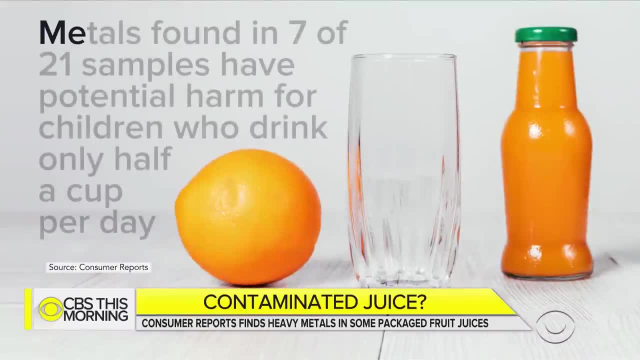 They found that every single product contained a measurable amount of at least one heavy metal, except for mercury. Twenty-one of the samples contained one combination of heavy metals that reached a level Consumer Reports researchers deemed concerning for daily consumption, And Consumer Reports says the metals found in seven of the 21 samples. 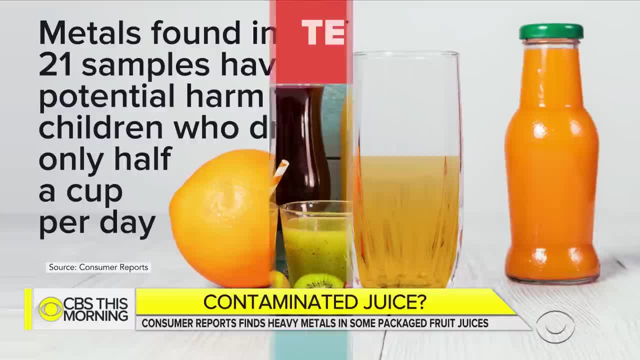 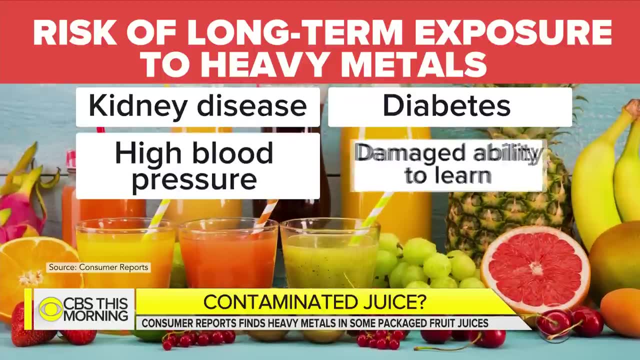 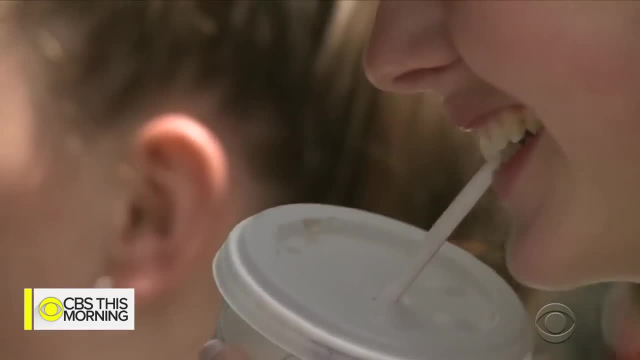 had the potential to harm children, who drink only a half cup per day. The CDC says long-term exposure to heavy metals may put people at risk for kidney disease, diabetes, high blood pressure, damaged ability to learn and certain types of cancer. Consumer Reports is recommending parents. 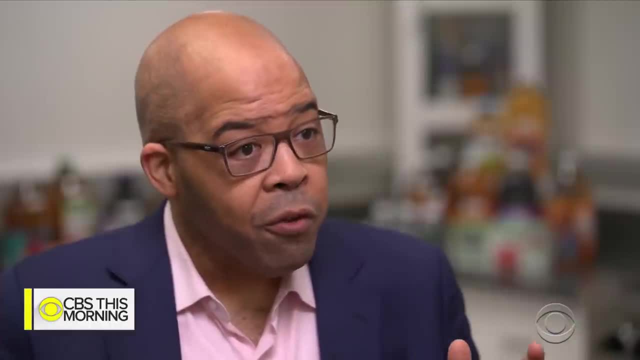 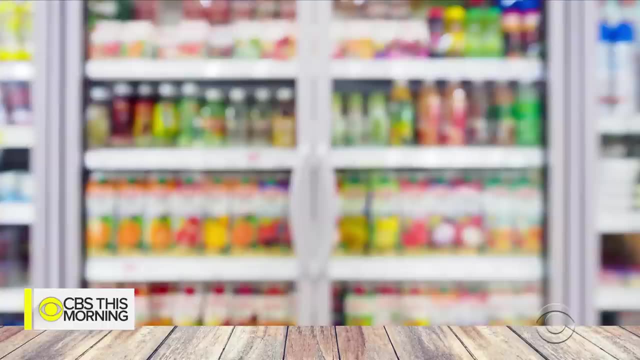 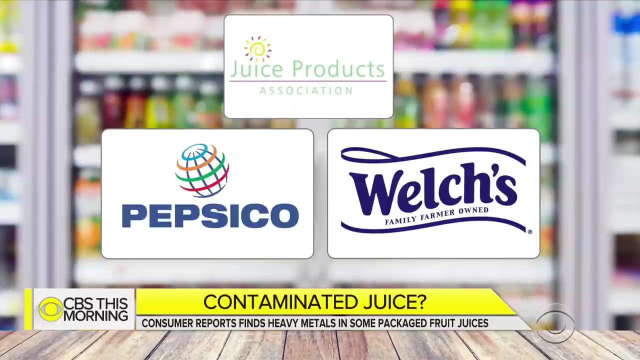 lower their consumption of heavy metals. So they should be concerned, but don't panic. Frequent exposure to these heavy metals through the juice is the concern. The Juice Products Association, whose board of directors includes executives from PepsiCo, Welch's and other juice brands whose products were tested, 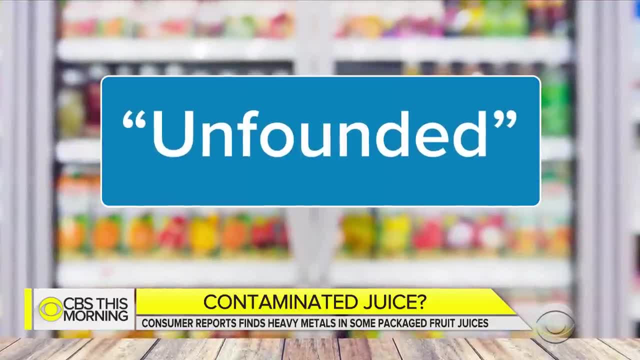 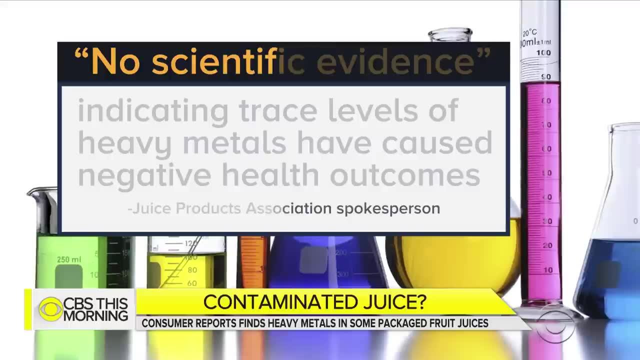 said they haven't seen the full study, but called the results unfounded and told us they're committed to providing safe and nutritious products that meet FDA standards. They also said there is no scientific evidence indicating that trace levels of heavy metals have caused any negative health. 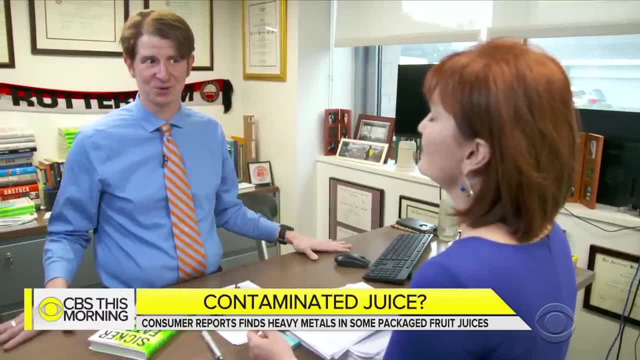 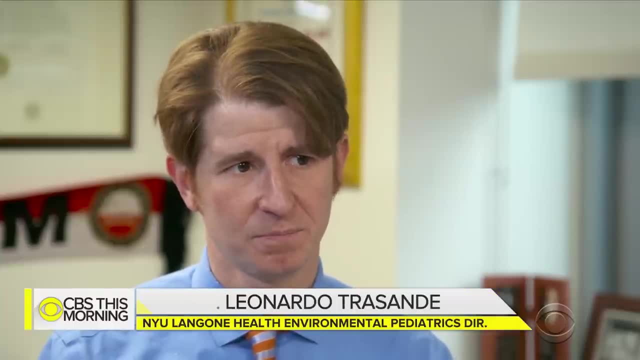 outcomes. But Dr Leo Tresonde, director of environmental pediatrics at NYU's School of Medicine, says: Dr Leo Tresonde, Director of Environmental Pediatrics at NYU's School of Medicine, says science is telling us increasingly that there are particular time points in life where even a small amount of exposure can disrupt. 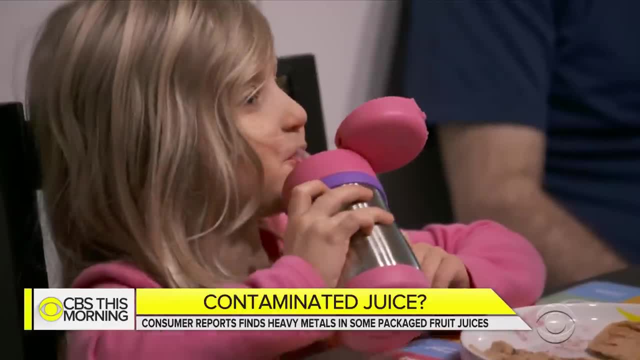 hormones and thereby contribute to disease. He recommends parents swap the juices for something else. Dr Leo Tresonde, Director of Environmental Pediatrics at NYU's School of Medicine, says My suggestion is to change the juices for something else. My suggestion is to change the juices for something else. Dr Leo Tresonde, Director of Environmental Pediatrics at NYU's School of Medicine, says My suggestion is to change the juices for something else. My suggestion is to change the juices for something else. Dr Leo Tresonde, Director of Environmental Pediatrics at NYU's School of Medicine, says My suggestion is to change the juices for something else. My suggestion is to change the juices for something else.